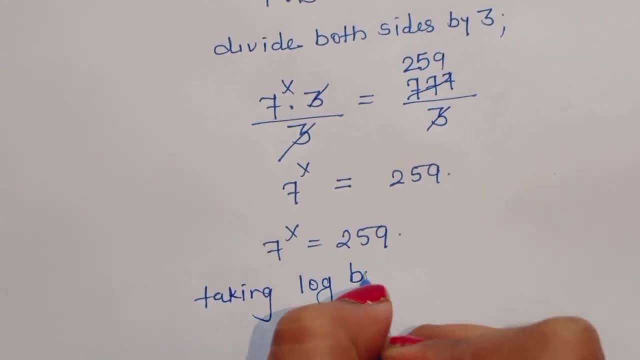 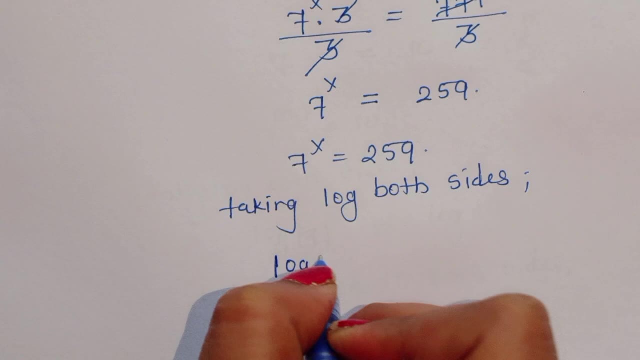 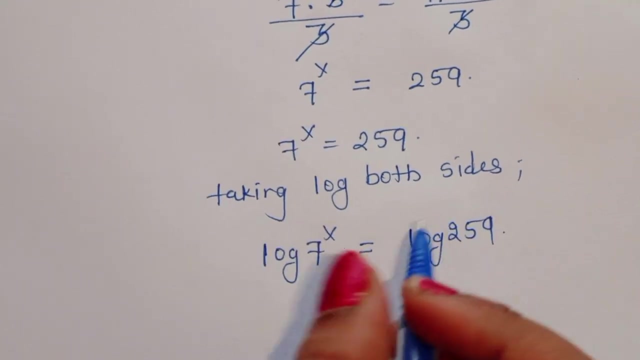 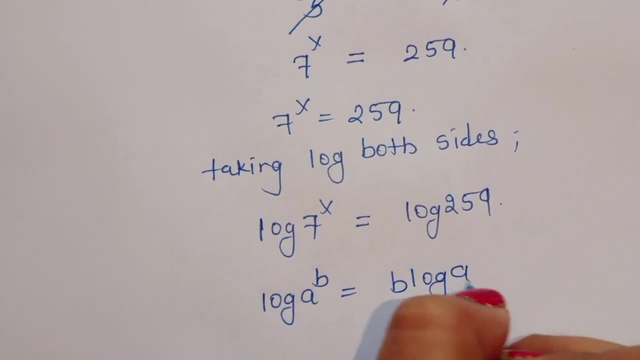 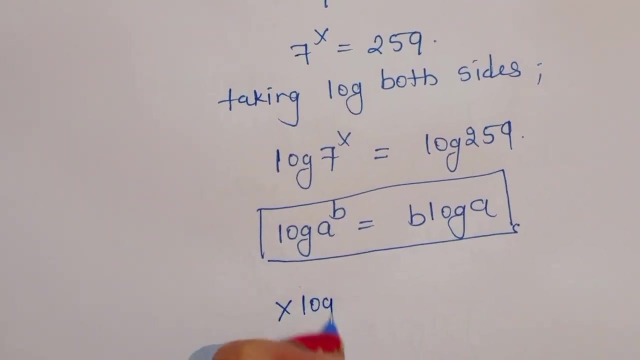 taking log here, then taking log both sides. Log of 7 power x is equal to log of 259.. Right, So we know the formula: Log of a power b is equal to b log of a. So using this formula here we will get x. log of 7 is equal to log. 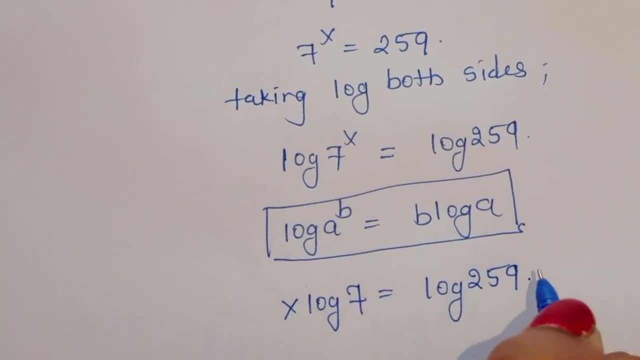 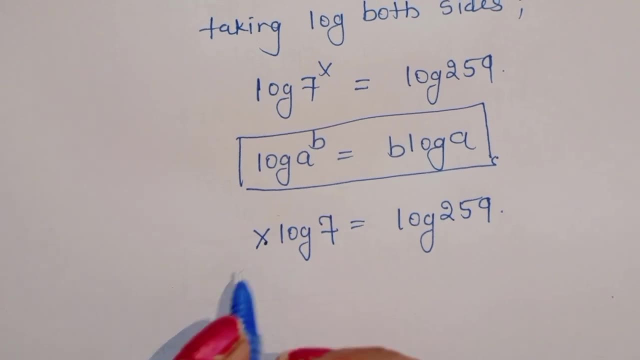 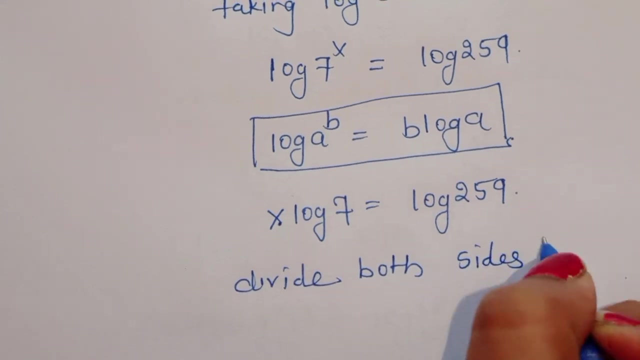 of 259.. Right, Type x- And here we are getting log of 7- is equal to log of 259.. Right, Then 7 power x. Right Now we can divide here by log 7.. So we will get value of x. So divide both sides by log 7.. 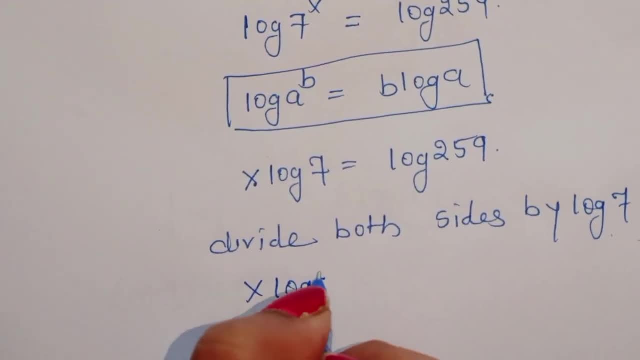 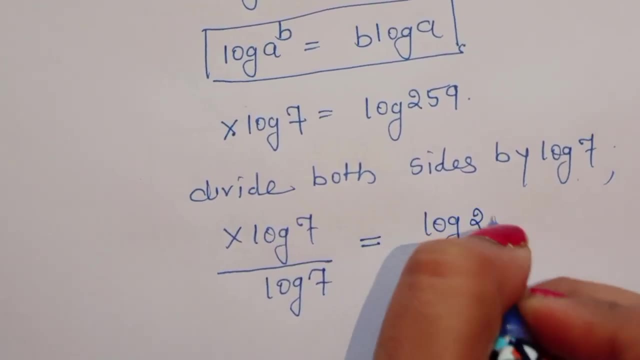 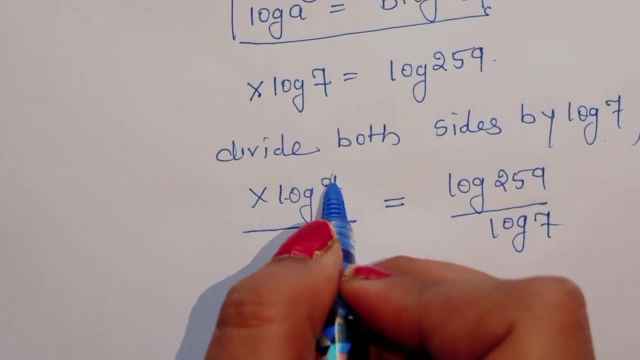 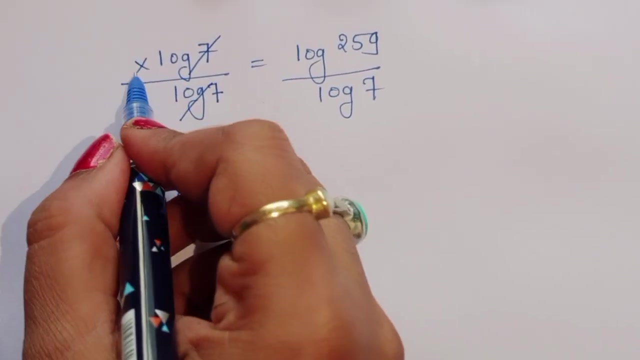 x log of 7 divided by log of 7 is equal to log of 259 divided by log of 7.. Right Now, x log of 7 divided by log 7.. So this will cancel here. Then we will get: x is equal to x is equal to log of 259 divided by. 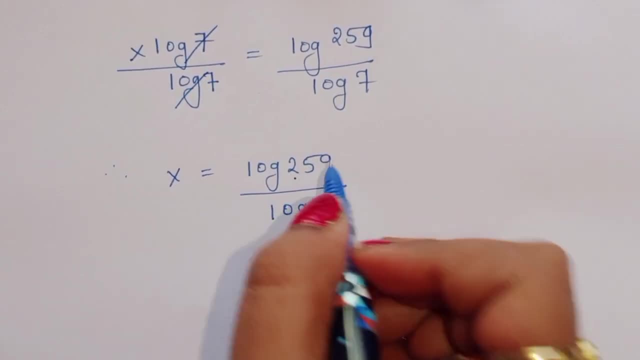 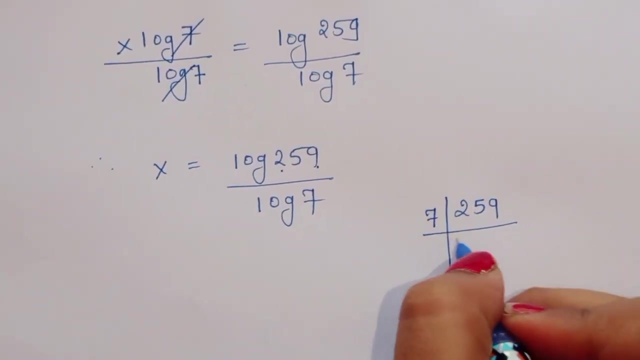 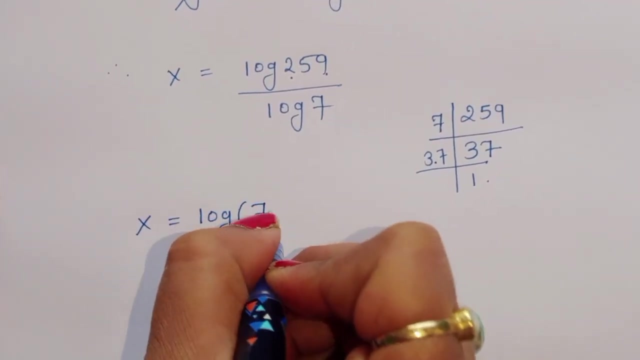 log of 7.. Now 259.. Factor of 259.. We can say: here 7: 3's are 21 and 7, 7's are 49. And here 37: 1.. So this is 7 times 37.. So we can say: here x is equal to log of 7 times 37 divided by, because. 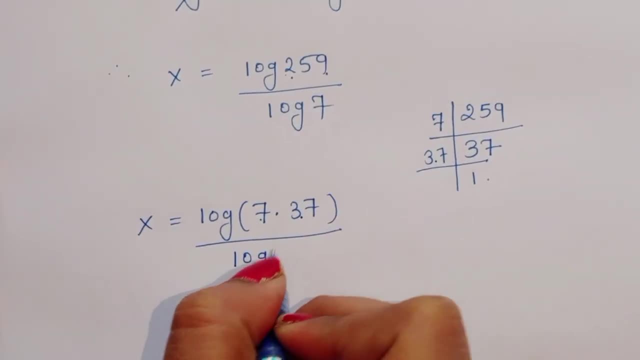 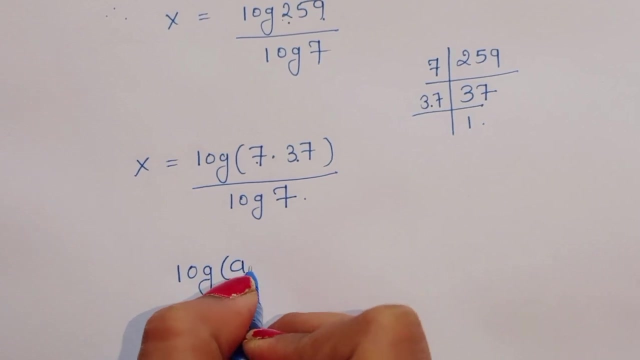 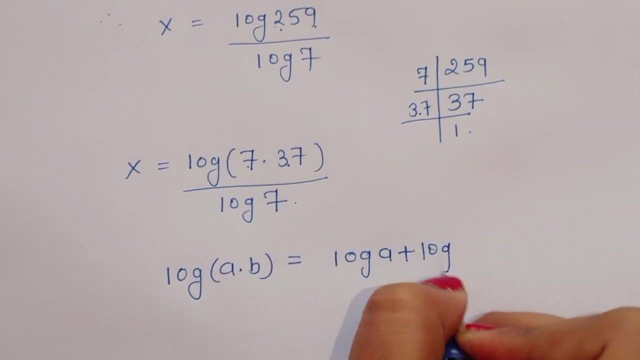 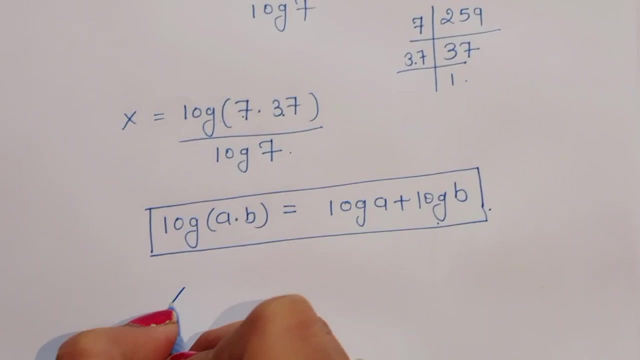 7 times 37, that is 259.. Log of 7.. Now we know the formula that is log of a times b is equal to. we can say it is log of a plus log of b. This is the log formula. So using this formula here we will get: x is equal to log of 7 plus log of 37.. 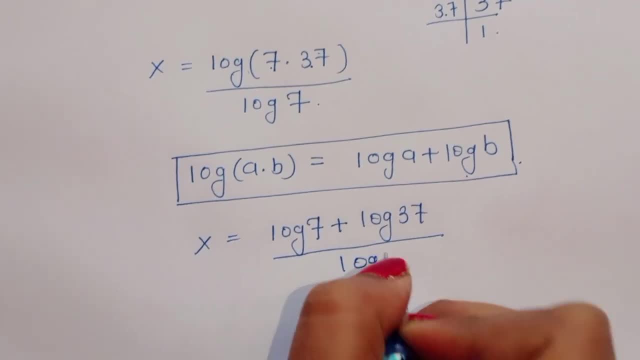 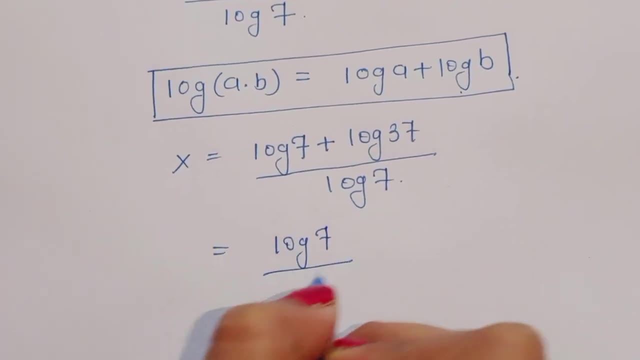 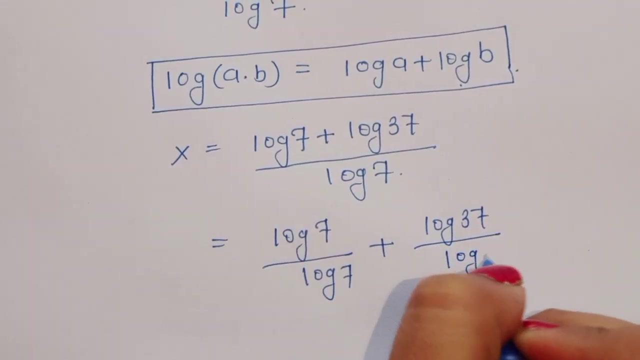 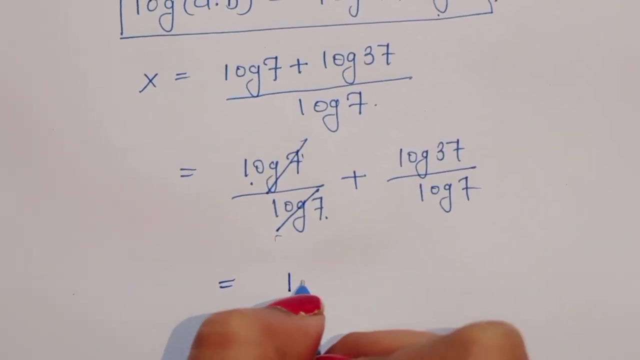 x. log of 7 divided by log of 7.. Right Now, separating term, then we will get here log of 7 divided by log of 7, plus log of 37 divided by log of 7.. Now, log of 7 divided by log of 7.. It will cancel. This is equal to 1 plus log of 37 divided by log of 7.. 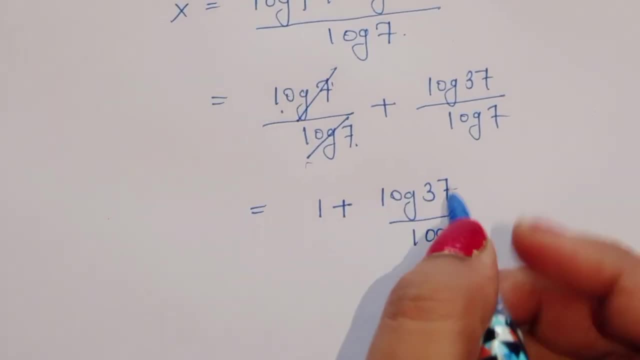 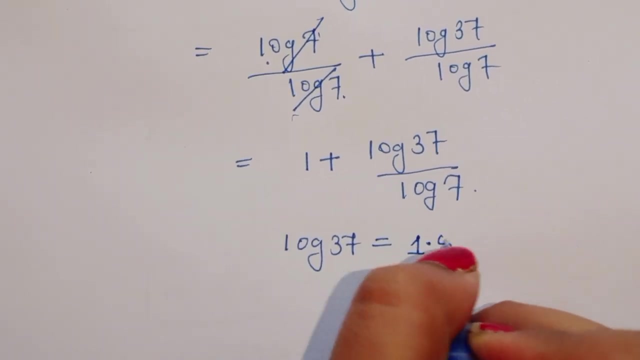 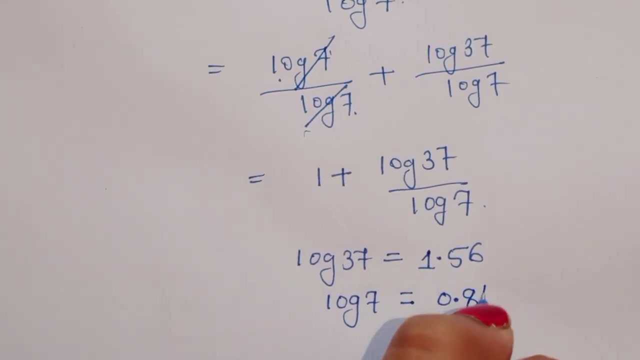 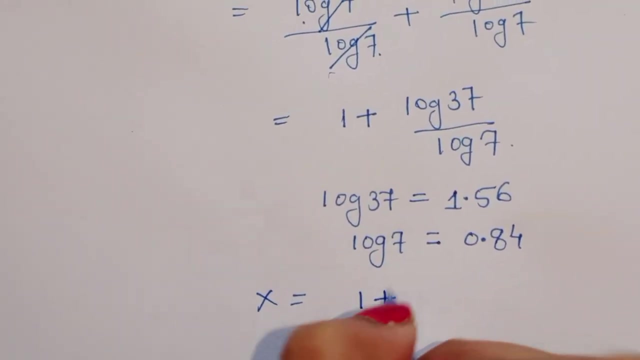 Now value of log of 37. Log of 37 is equal to- we can say it is 1.56.. And log of 7 is equal to 0.84.. So we can say: here is equal to x, is equal to 1 plus log of 37, that is 1.56.. 1 plus 5, 6.. 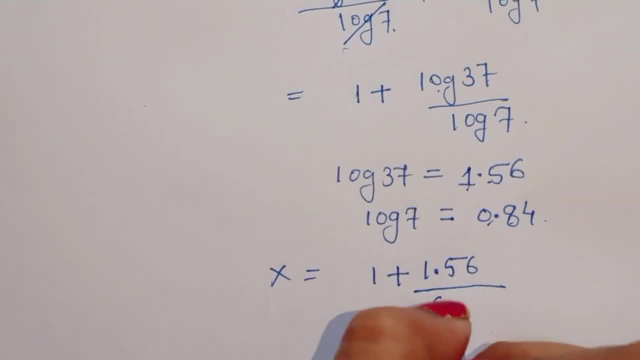 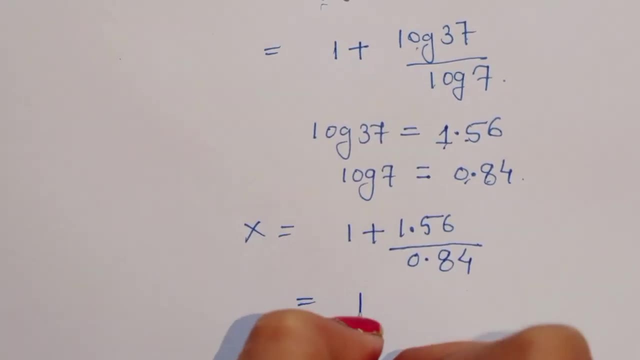 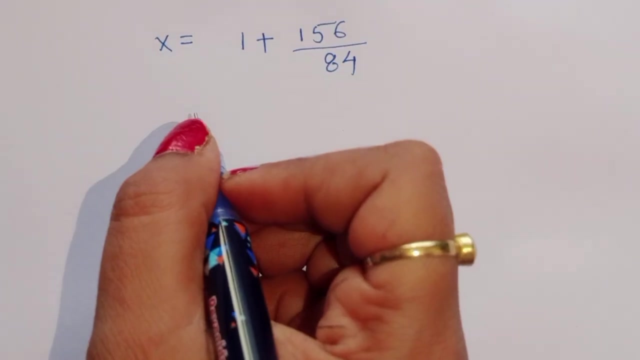 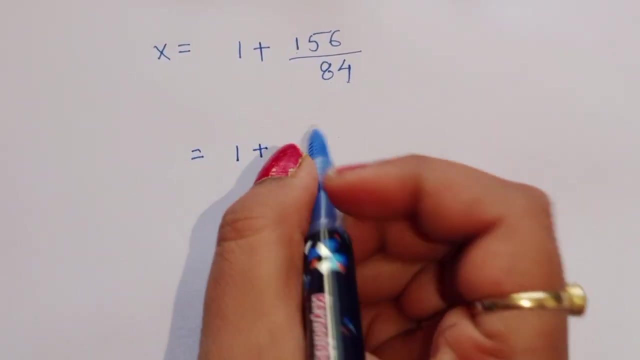 1 plus 5, 6 divided by 0.84.. 0.84.. Now, multiplying both side by 100, then we will get here: is equal to 1 plus 1.56 divided by 84.. Is equal to 1 plus Now, when we are dividing this 1.56 divided by 84, then we will get here 1.85.. 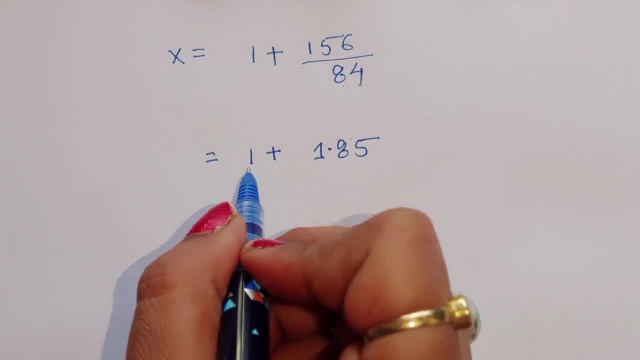 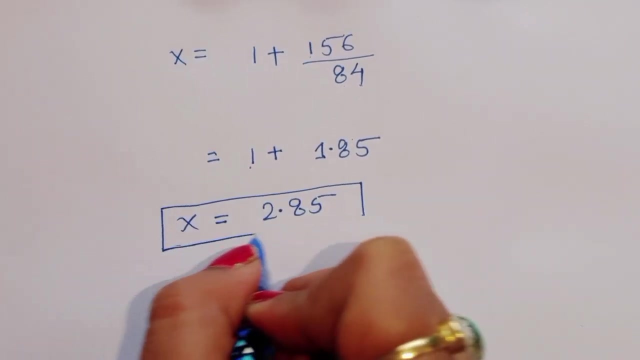 1 plus 1.84.. 1 plus 1.85 is equal to. we can say 1 plus 1, that is 2.85.. Value of x is equal to 2.85.. And this is solution. Thank you. 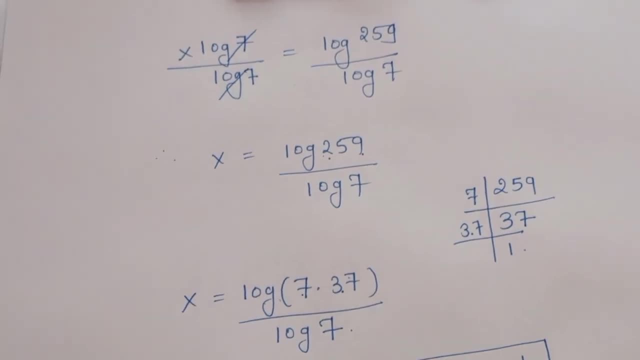 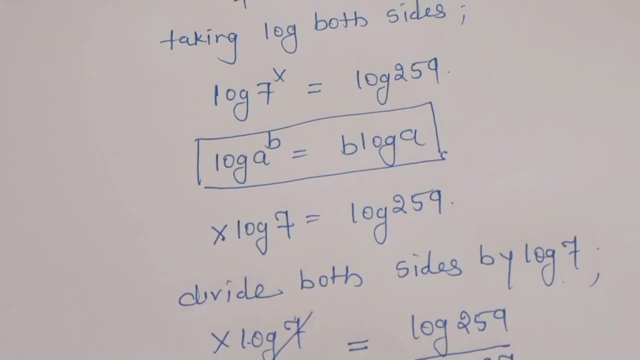 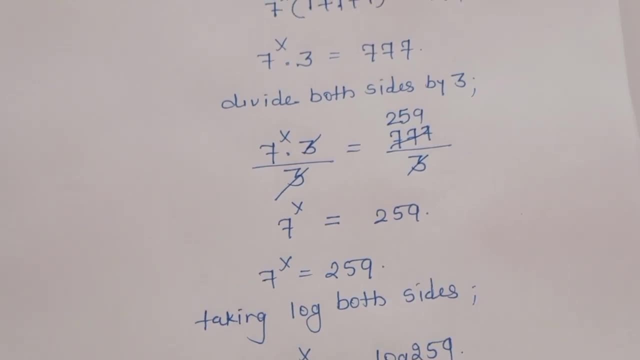 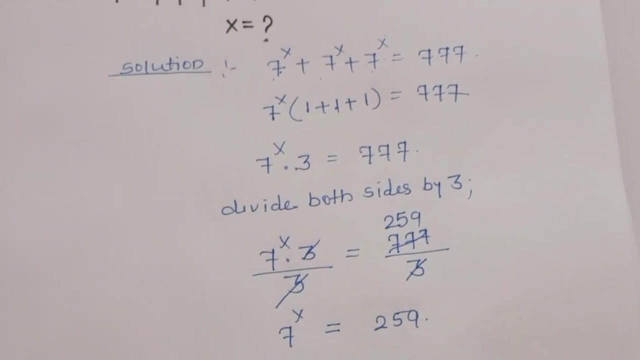 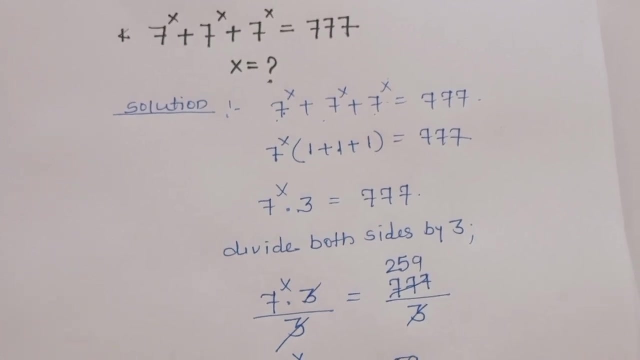